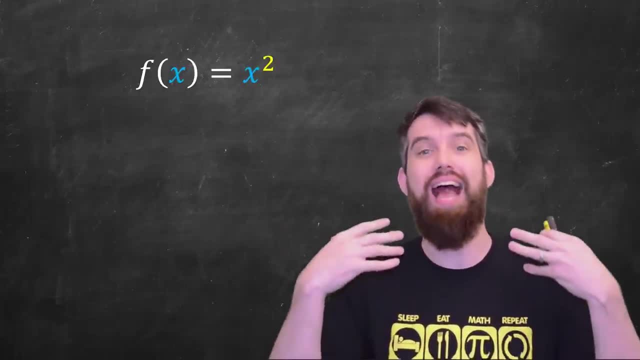 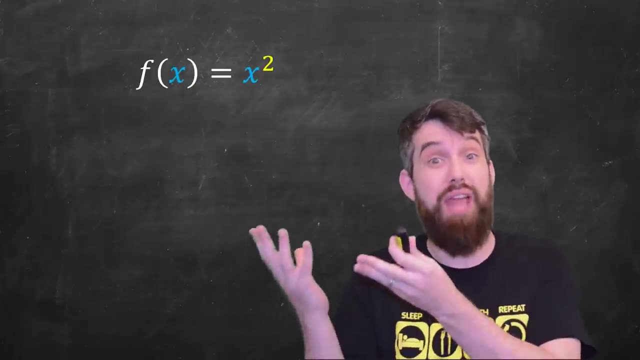 Well, I think a function is sort of a transformation. There's some inputs and the inputs are transformed And it's formed into being some outputs And in the case of something like f of x equal to x squared, the kind of function you'd see in first-year calculus, that you have a one-dimensional. 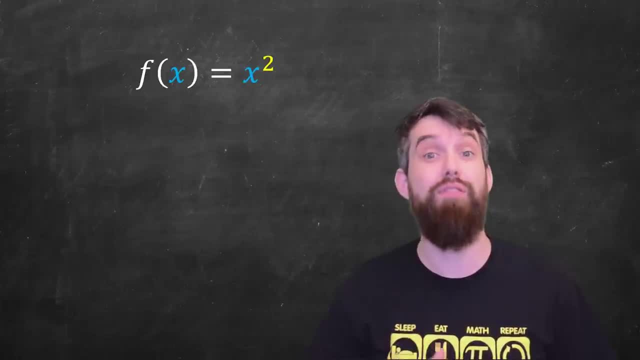 input x and a one-dimensional output f of x. However, we can imagine our transformations being in higher number of dimensions, where the inputs might be a whole bunch of different variables and the outputs might be a whole bunch of different variables And one way. 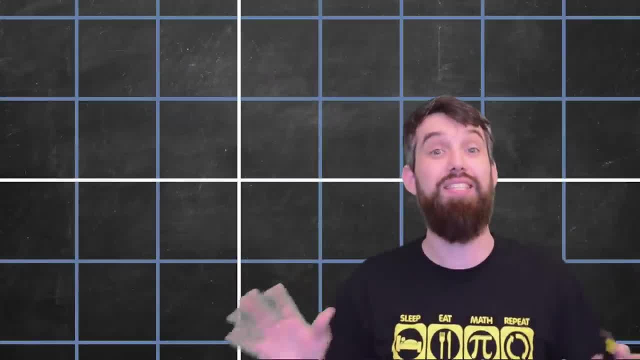 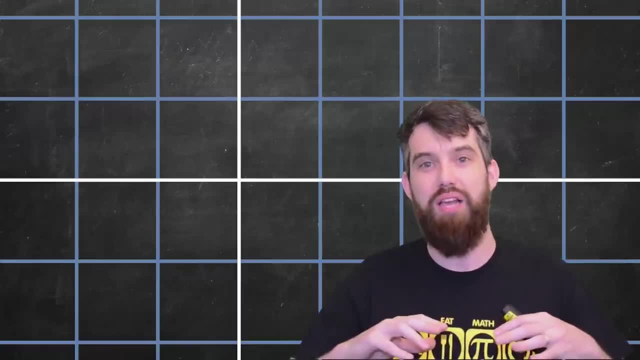 you can visualize. this is the following. So I'm going to show you this here. This is going to be the two-dimensional plane, and I've got my origin over here. Now, a way that I can view a transformation that takes the plane and transforms all the points to other points on the plane is just by showing 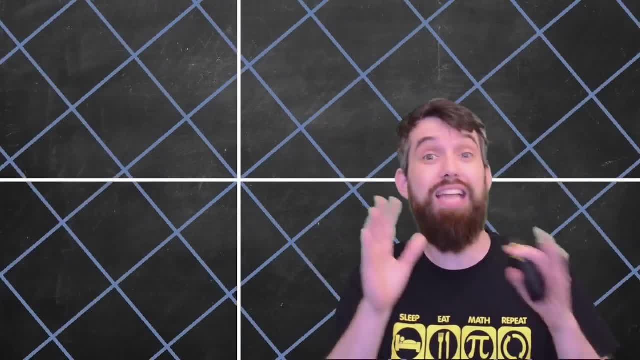 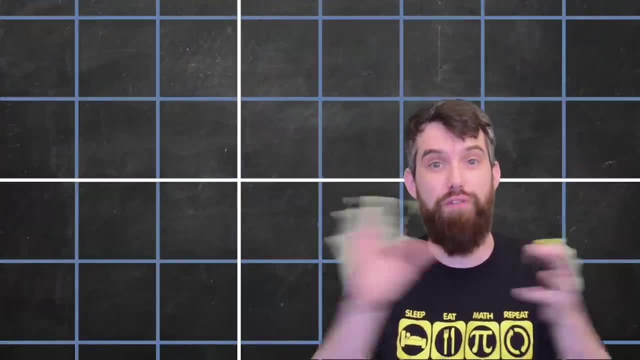 you how they move. So, for example, this is just going to be the rotation of the points on the plane by some number of degrees. Or I could have a different one. I could take this one that takes all of the plane and it just compresses it down, It makes it a. 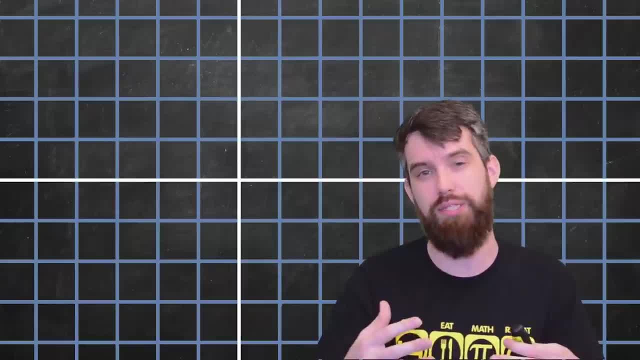 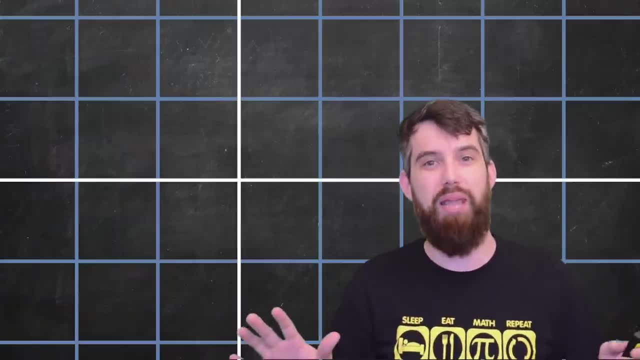 factor of two closer together for any pair of points. Okay, I can do all sorts of different transformations from the plane to the plane. What about this one? that's a little bit funky. So this one that starts with my plane and then just goes off in some kind of crazy direction. 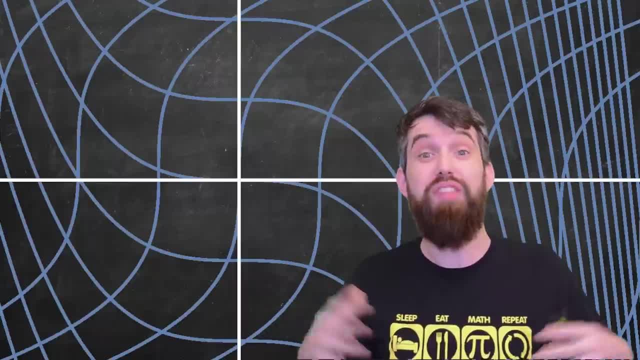 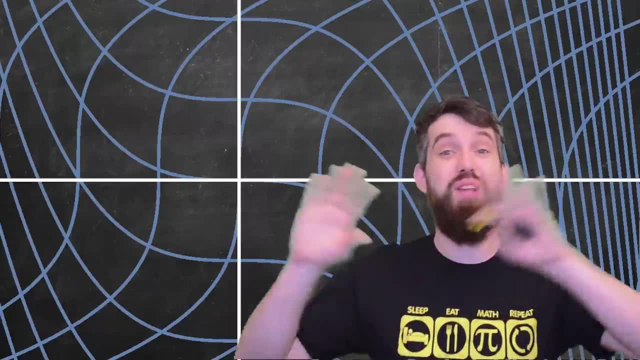 out like this And it looks pretty cool, but all of these are transformations from two-dimensional space to two-dimensional space. Now, as you can see, these very quickly get really, really complicated, And while it's true that you can study them, you can't really do anything about them. 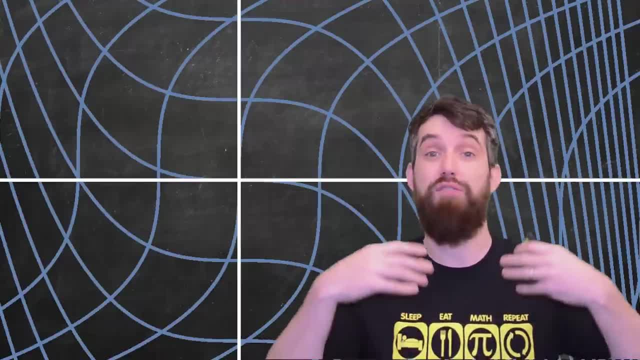 So you can't really do anything about them. So you can't really do anything about them. However, you could study them in a variety of ways. For example, if you study multi-variable calculus, you would look at these transformations, but you would impose some condition. For example, 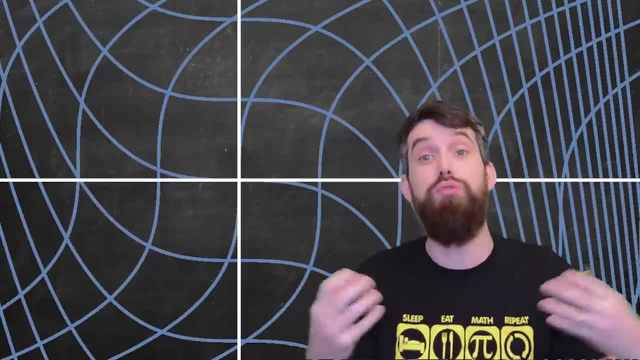 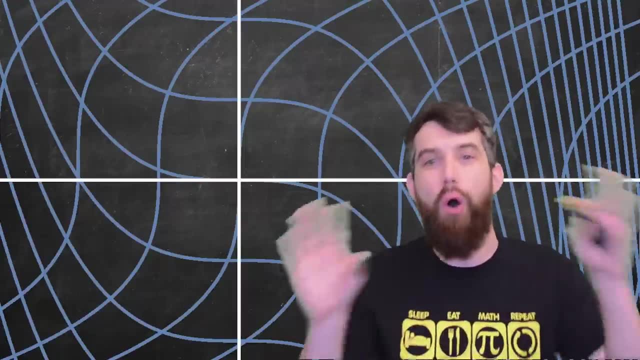 you'd impose perhaps that these functions were smooth transformations, differentiable transformations in some sense. But in our course in linear algebra we're going to demand a lot. We're not going to look at all the transformations, We're going to look at specific ones And the two things. 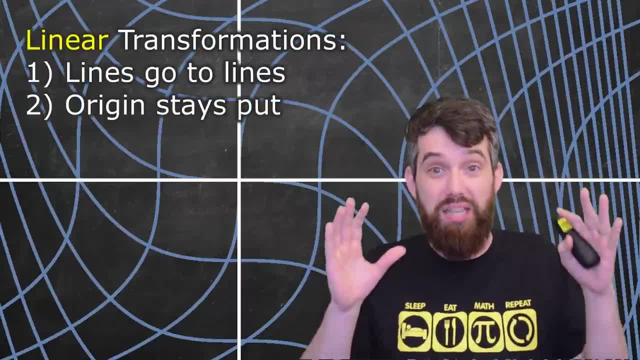 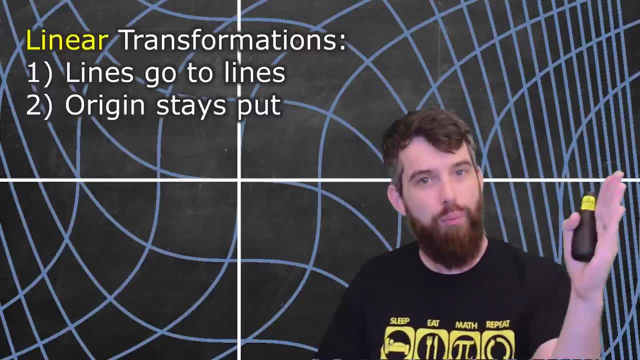 that we're really going to demand are: first of all, we're going to demand for a linear transformation 1. we see here, If you start with a straight line, then you're going to end up with a straight line. And secondly, if you start right on the origin, no matter what your. 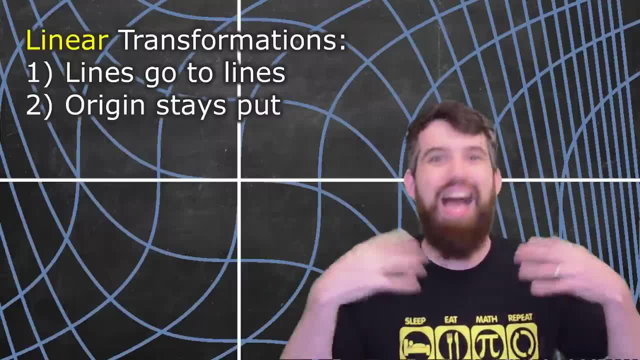 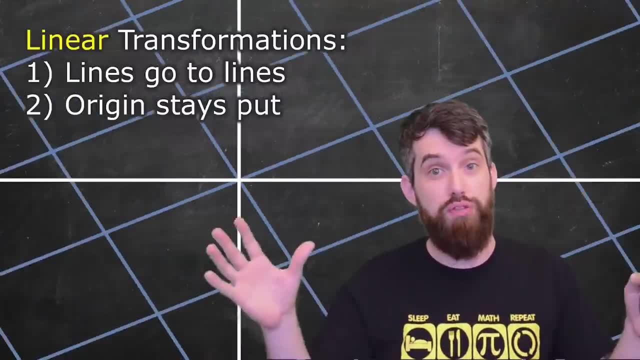 transformation does? it takes you right back to the origin. That's the kind of transformation I'm going to consider, So this one doesn't apply, but this is an example that does work. Starts with lines, moves it around and you get some. 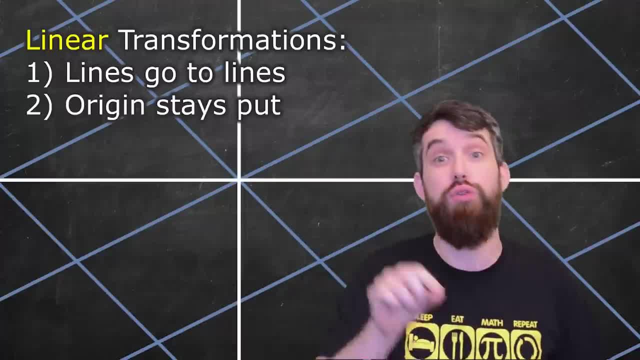 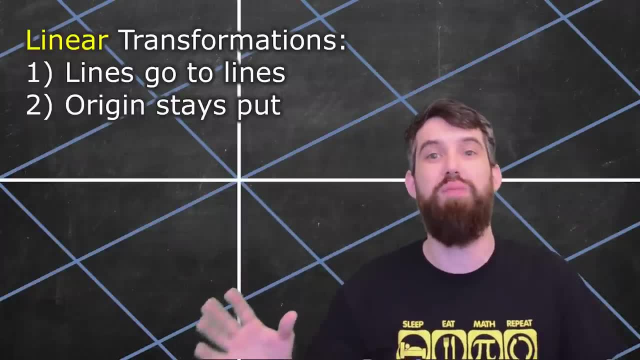 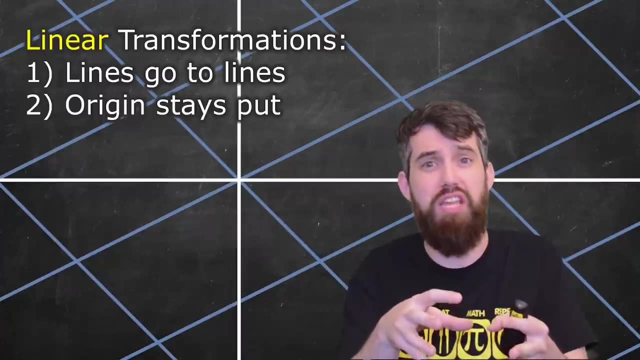 other lines. So this does take lines to lines. it takes the origin to itself. I'm being pretty restrictive here. A whole large number of transformations- Way more transformations, are not linear than these linear ones. It's quite a restrictive set. So if I'm going to narrow my focus into a relatively 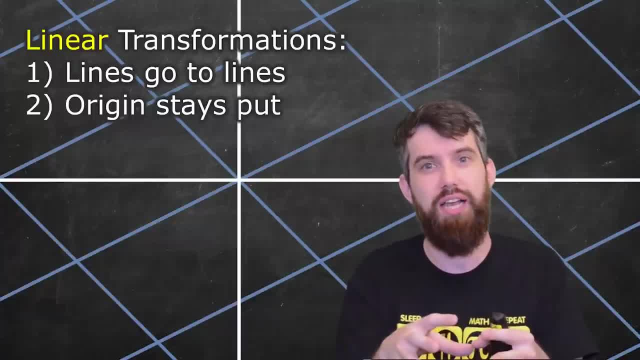 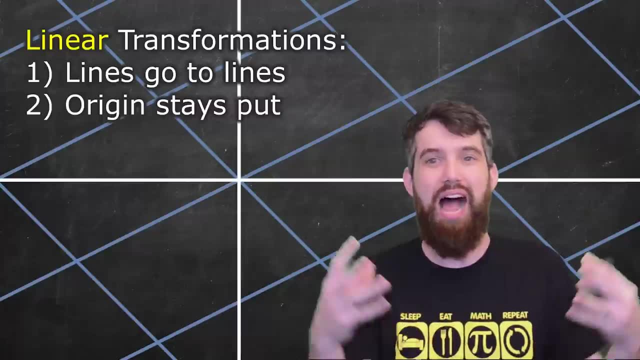 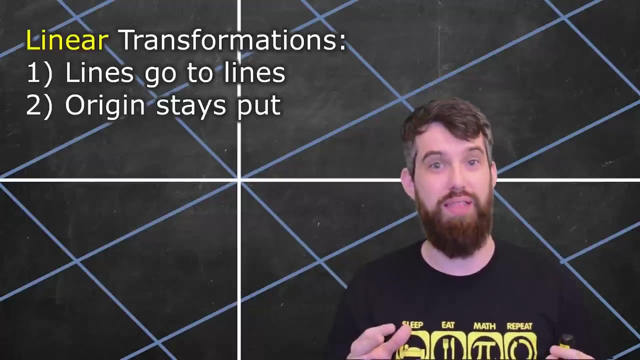 restricted set of all possible transformations, then I have to get something out of it. I have to say that, well, these linear transformations are really nice, really easy, really powerful, that I am worth spending a lot of time focusing on this restriction. And indeed that's the case. Linear algebra, that is. 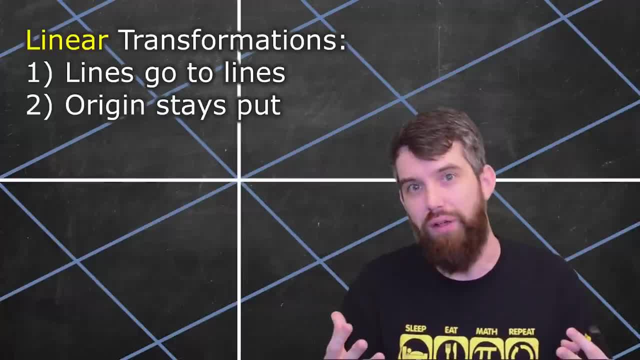 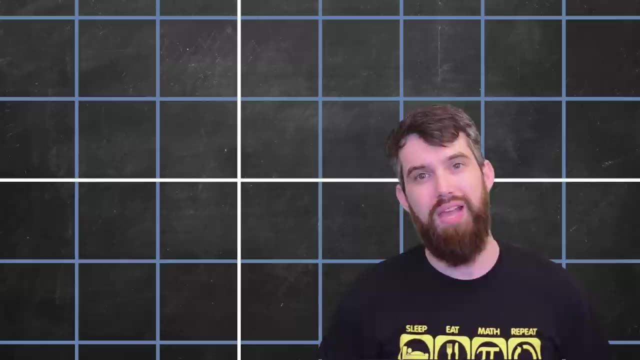 the study of these linear transformations is so powerful that the the restriction you make, demanding that lines go to lines and the origin state put, turns out to be worth it. So let me show you some ways where this is going to work. The first thing I want to note is, if I have my standard grid, I'm going to put two arrows. 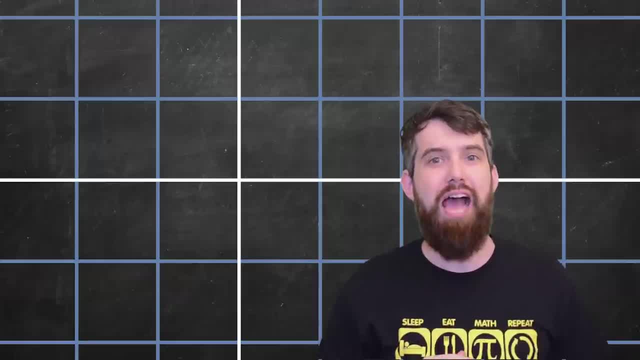 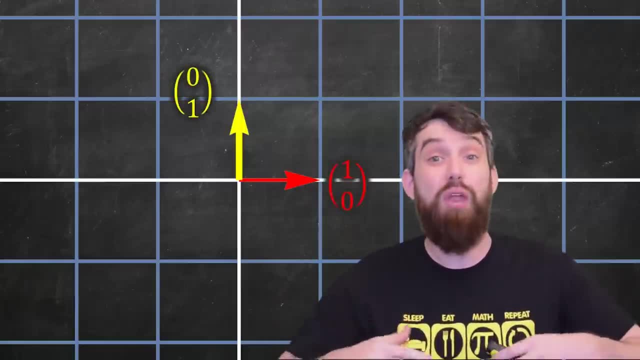 — you might know the term vectors for them, but we'll call them arrows here — and these are going to be very standard arrows. The red one is going to start at the origin and go over to the point, and the yellow one is going to start at the origin and go up to the point. 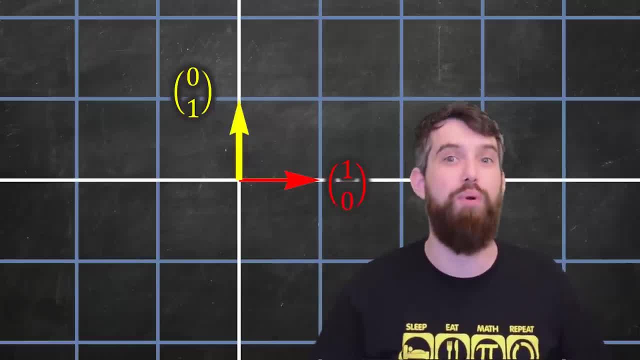 When I read them vertically, I mean something like one to the right and zero up, or zero to the right and one up is what I mean by this vertical placement of numbers. Okay, so I have these two little arrows and let me apply my transformation. 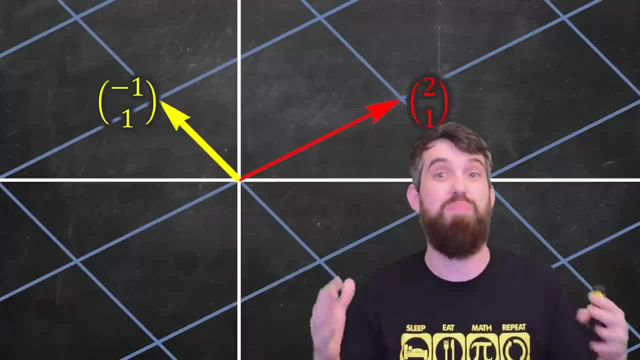 They're going to go off and do something. They're going to move somewhere else. and because I've pruned it in, I can see here that the yellow one denotes going one to the left and then one up, and that the red one 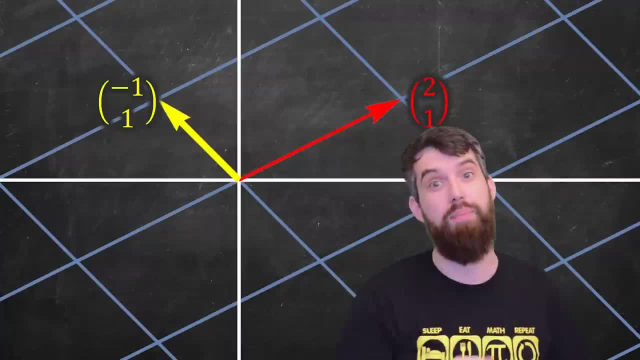 is going to denote going two to the right and one up. So I know where those two end up. I know where the red arrows are going to go: the standard red one, the standard yellow one. But what about some other arrow? What about this funky one that we have down here? 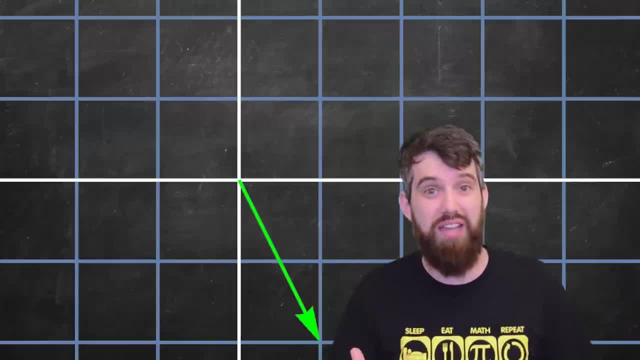 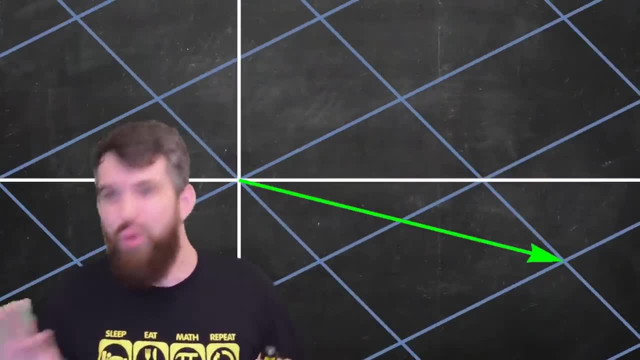 Well, this one. I can think of it as going one to the right and then two down, okay, And I could go and apply my transformation. it's going to move off somewhere, but what are the coordinates of this? Where actually is this gone? 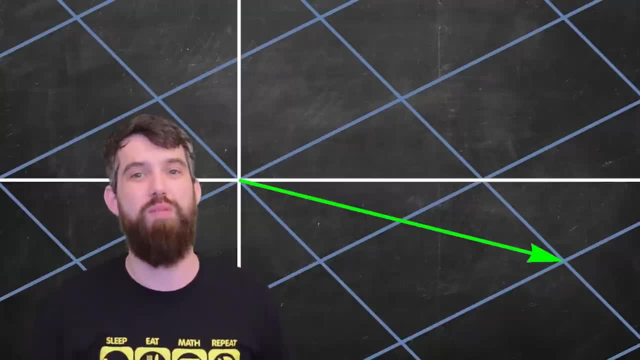 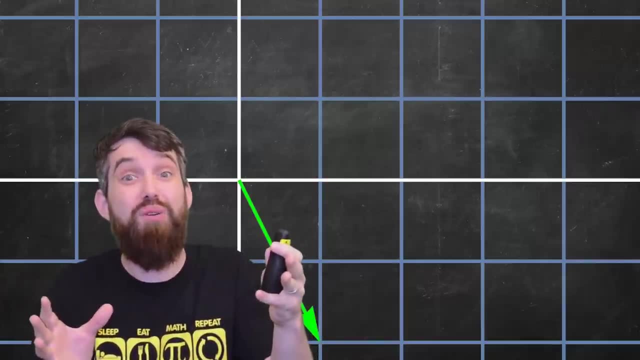 Now the whole magic, the whole wonderful part about linear algebra is that if I know where the red and the red are, I can go and apply my transformation And the yellow arrow go- those standard arrows- I can figure out where all the other vectors. 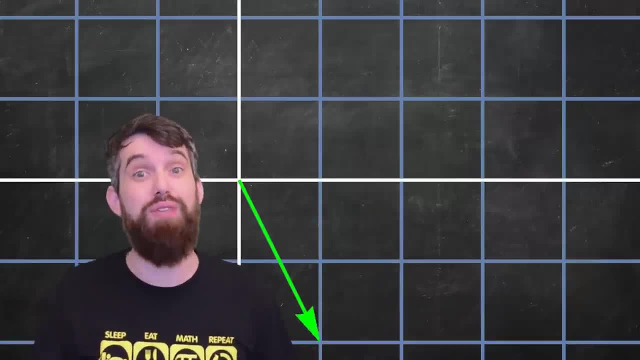 are going to go as well. Look at this: this is one to the right and two down, so how would I just go and put those vectors in The red one denotes my one to the right, and then for my yellow one. I haven't done the. 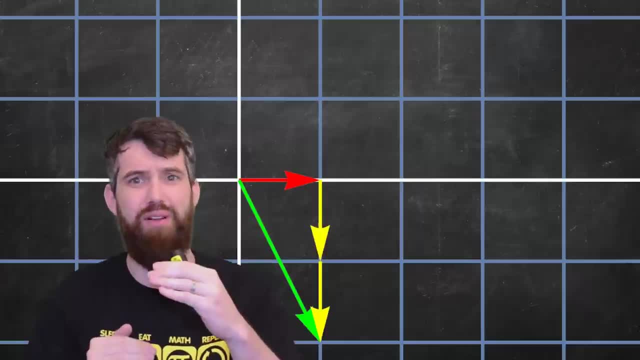 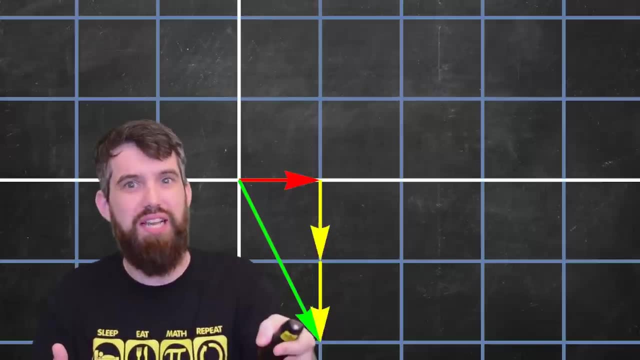 arrow pointing up. I've done the arrow pointing down, which is kind of like a negative of it, but either way it means to step down one. So then this green arrow is really like doing the red arrow first and then negative two of the yellow arrows. 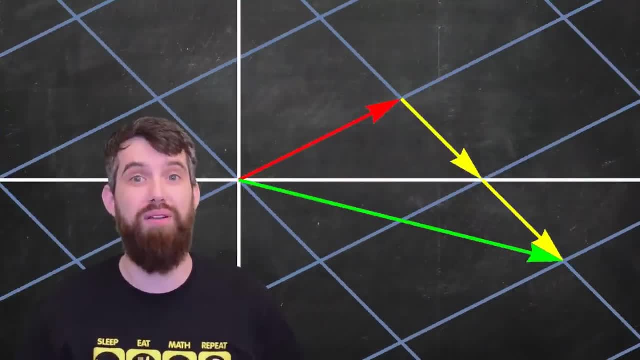 And then if I go and transform this, okay, this goes off somewhere, and one of the nice things about our condition that lines have to go to other straight lines- is this triangle that we formed. it goes to some other triangle, But now I can figure out what the coordinates of this green arrow are, because I know what. 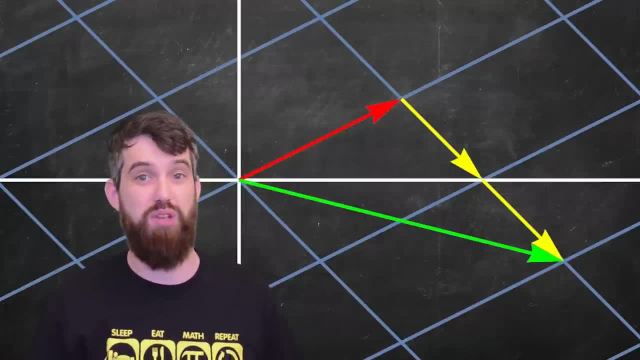 the red arrow did, and I know what the yellow arrows did. The red arrow that started as one zero. one to the right and zero up. it transforms to two to the right and one up. Meanwhile, the yellows in the negative direction are going to denote one to the right and 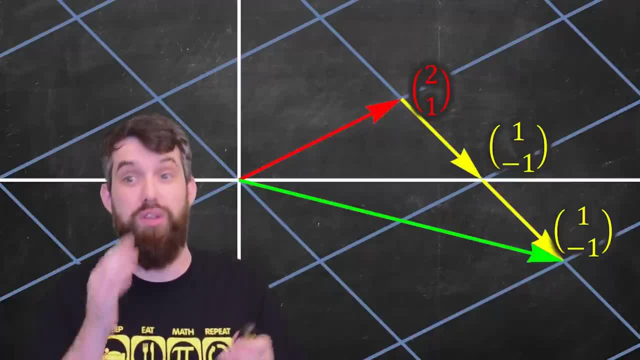 one down and I got two of them, And so, putting this together, if I just look at what's going to the right, well, I have two to the right, one to the right, one to the right. that ends up four to the right. 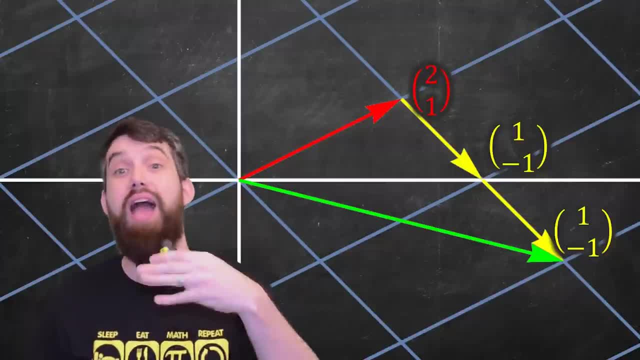 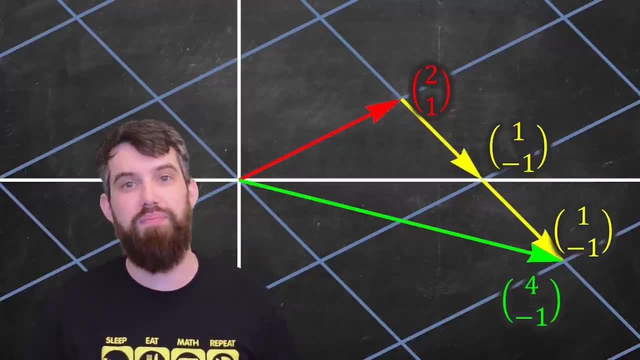 If I think about up down, well, first I'm going to go one up, one down and another down. So what do I have? This particular point four minus one, Four to the right and one down. And I can even take these and sort of make it into sort of an equation of some form. 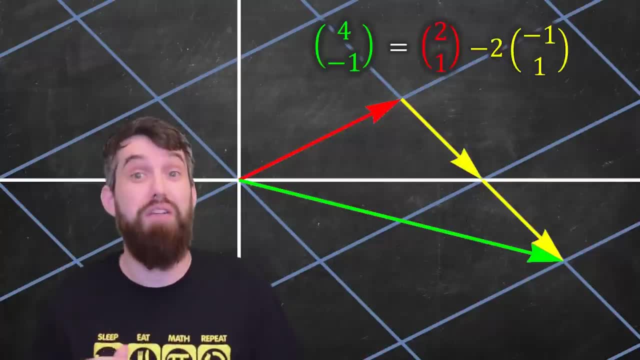 So let's put them all together, And so what I get is that this four minus one, four to the right and one down, is written as wherever the red arrow is, Okay, The red vector is going to go the red arrow, two to the right and one up, and then I subtract. 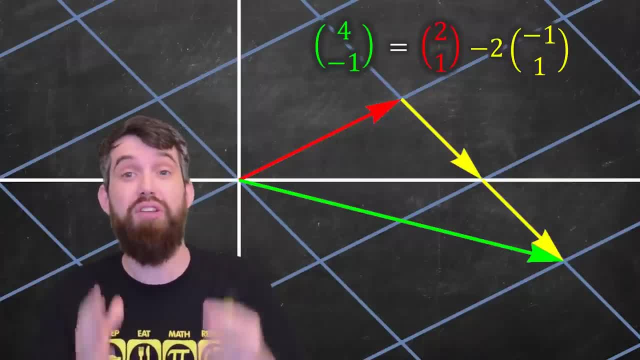 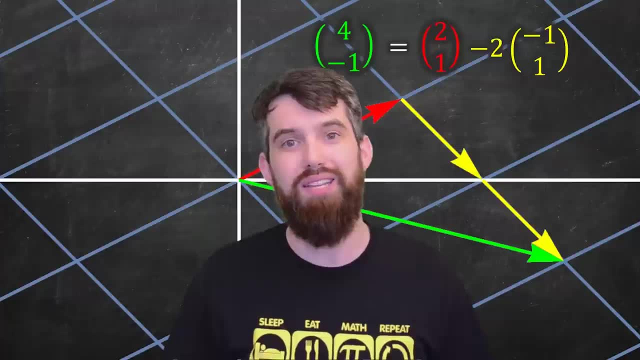 off two, subtracting because the yellow arrow is in the other direction. I subtract off two of these vectors, that are the one to the left and the one down, And so I have this nice little algebraic formula for it. So what's the key lesson? 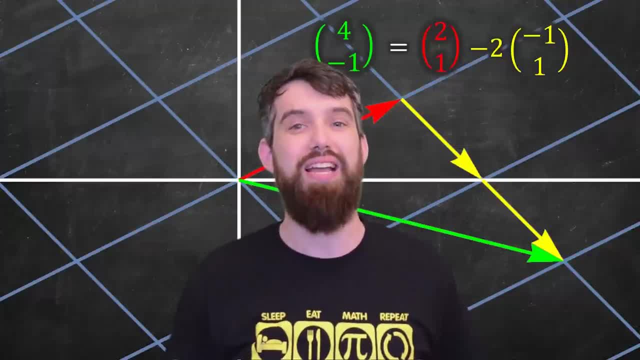 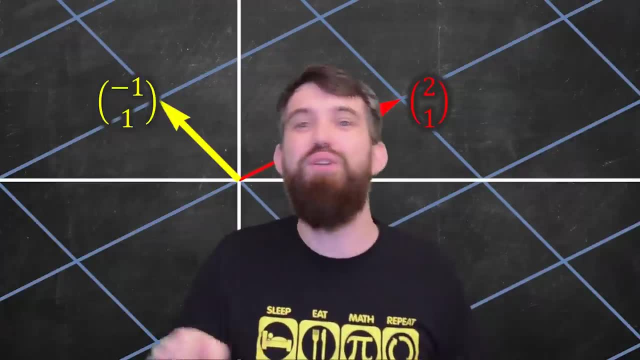 The key point is that if I know where the original red and yellow arrows are going to go- in this case they go to the two one and the minus one one- if I know where those go, I can figure out any other vector And the entire plane, because it's just going to be written as some combination of the red. 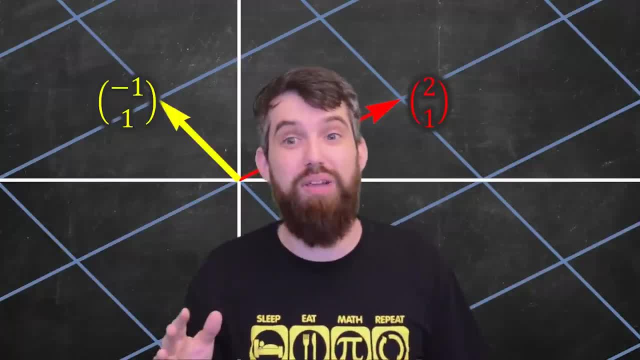 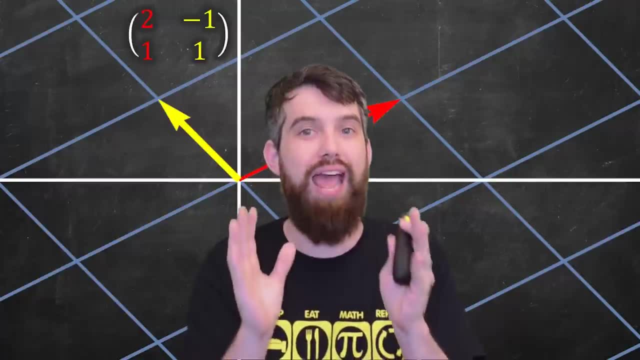 and the yellow vectors. So all that matters for my entire transformation is knowing where the red and yellow vectors go. They go here. So I'm going to combine this information that I've got separately. I'm going to put it together into one algebraic thing we call a matrix, where the columns of this so-called matrix 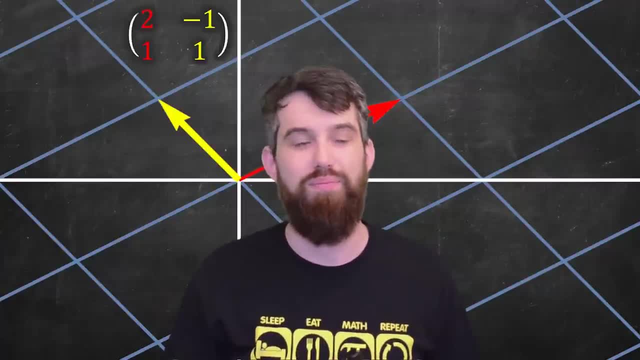 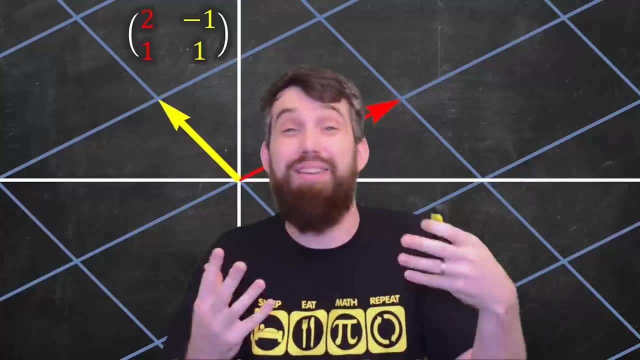 denote where the red goes and where the yellow goes. By the way, I'm doing from two dimensions to two dimensions. You could have three dimensions to two dimensions, Or three dimensions to eight dimensions, Or eight dimensions to a hundred dimensions, All sorts of different possibilities. 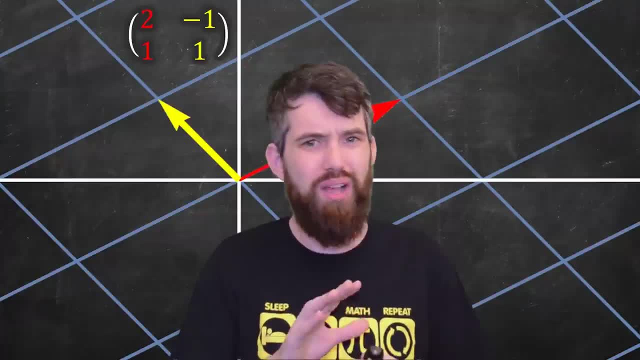 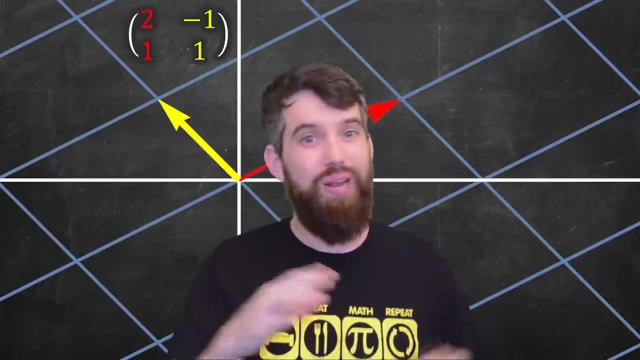 I'm just visualizing it in two dimensions. So what we've really learned here is that for these linear transformations that take lines to lines and the origin to the origin, that really they are defined by only these four numbers. And if you know those four numbers you can figure out the entire transformation. 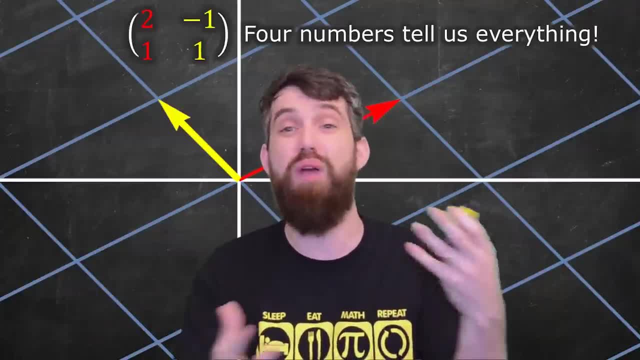 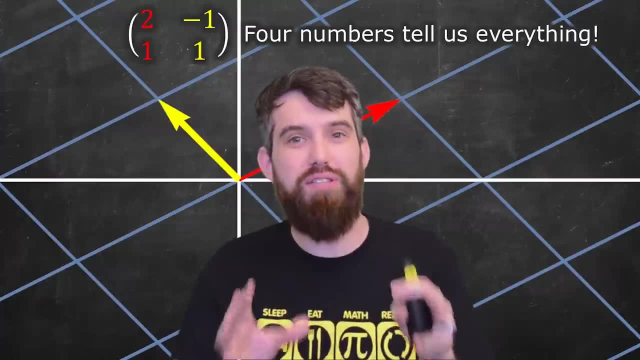 Any other point. you just try to describe it in terms of the red and yellow vectors. This tells you where the red and yellow vectors go. That's all you need to know. So This is just the start of scraping the geometric picture. 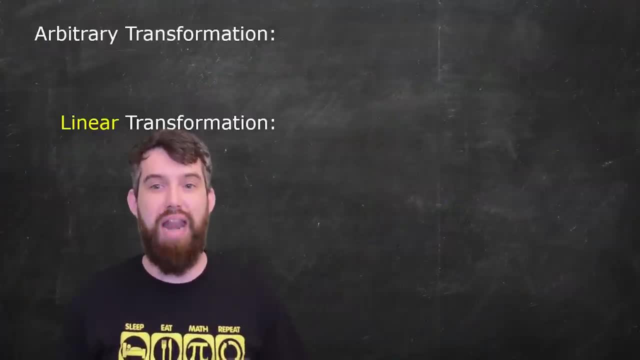 What about the algebraic picture? So let's just get rid of everything for a moment. And I want to compare what I'm going to call an arbitrary transformation and a linear transformation. So the idea here is that if I'm going from two dimensions to two dimensions that I've 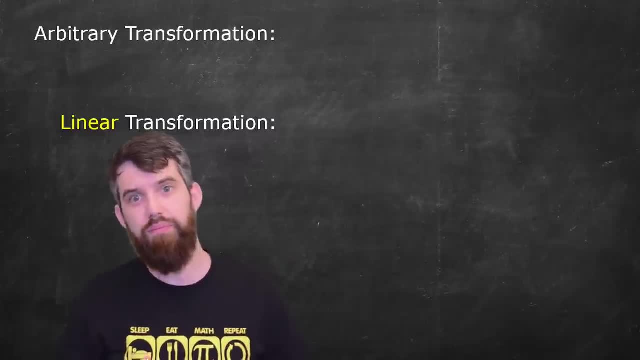 got two input variables, x in and y in, and I also have two output variables, x out and y out, And that they're related in some way, That the x out is just going to be some function. that depends on the function. And that the x out is just going to be some function that depends on the function And that the x out is just going to be some function that depends on the function And that the x out is just going to be some function that depends on the inputs. 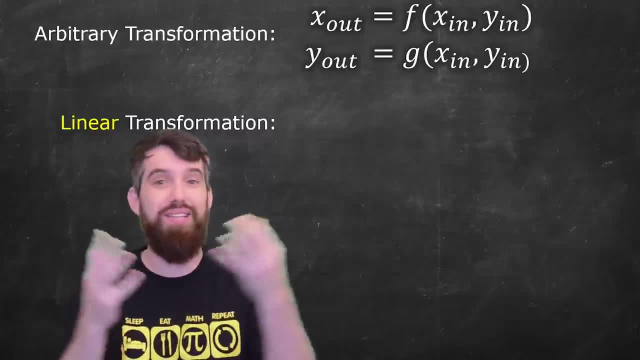 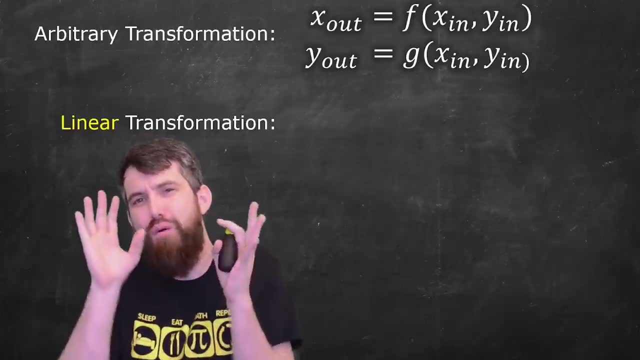 And the y out is just going to be some function that depends on the inputs. I don't know exactly what they are, but they're just some arbitrary function. But again, we're not looking at all transformations. We're going to focus our attention to what I'm going to call the linear transformations. 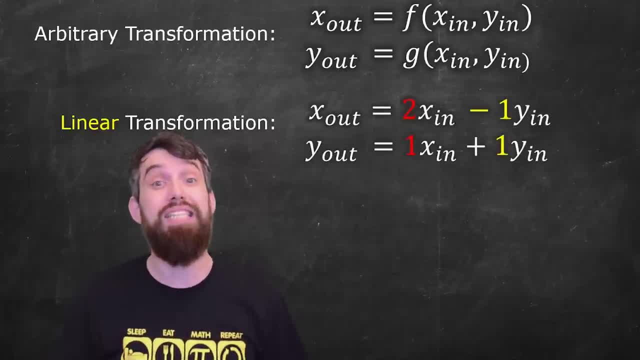 And a sample linear transformation looks like this: I've given an explicit function for what the f and g are. They are a so-called linear combination And the key thing about these expressions are that any input variable, Like the x in or the y in. 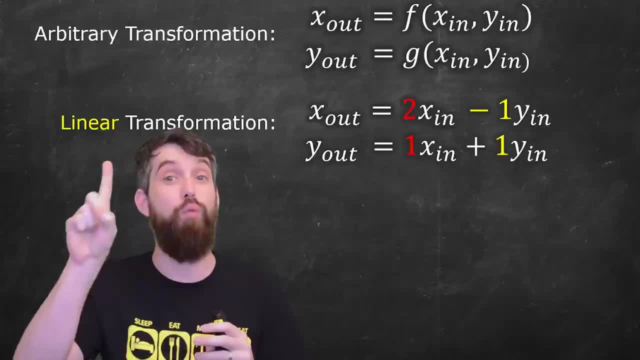 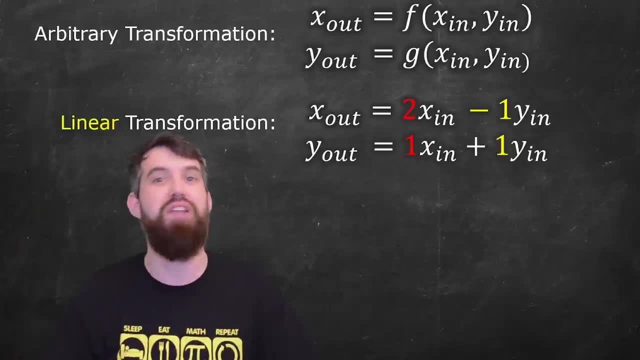 It only appears in the expression raised to the power of 1.. That's my algebraic constraint. I don't have any x in squareds. I don't have cosine of x in. I don't have the square root of x in. 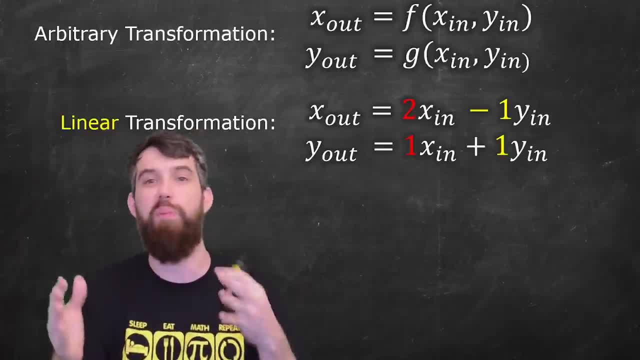 I have x in to the power of 1 and y in to the power of 1.. I'm allowed to multiply by some scalar constants like the 2 and the minus 1.. That's it. It's a pretty imposing restriction, But when you get that imposed restriction, 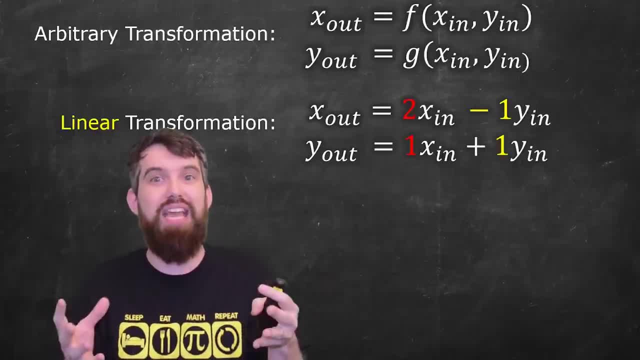 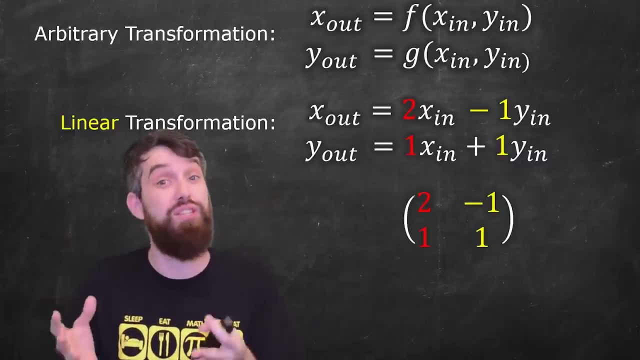 Then These types of linear transformations again are defined by these four numbers, And so again I can sort of associate this one thing I'm calling a matrix as the key thing that describes this algebraic description, And indeed those four numbers are going to tell us everything. 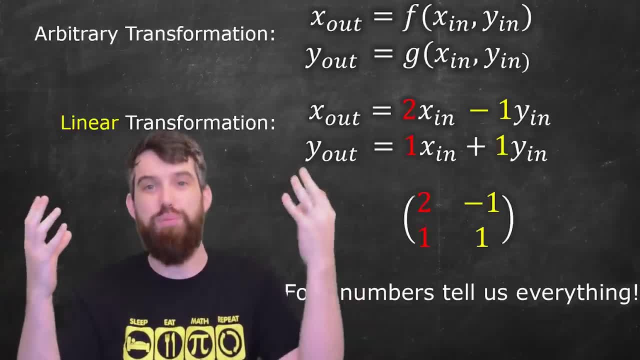 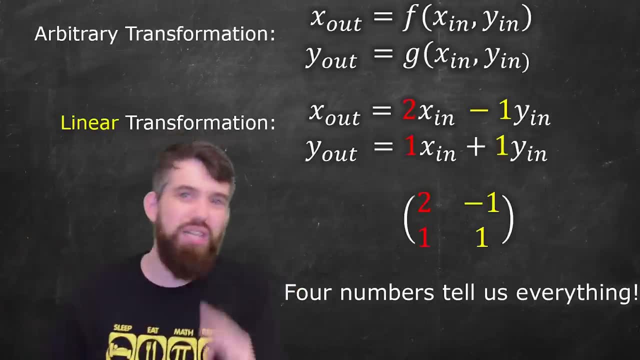 So, in other words, we have this geometric world, We have this algebraic world And we have different types of constraints. The transformation, the geometric world was imposing that a straight line has to go to a straight line and the origin to itself. 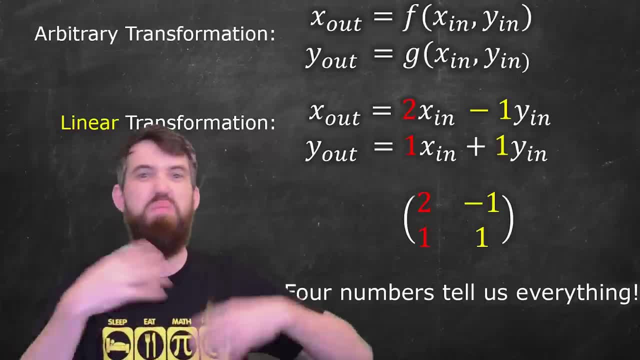 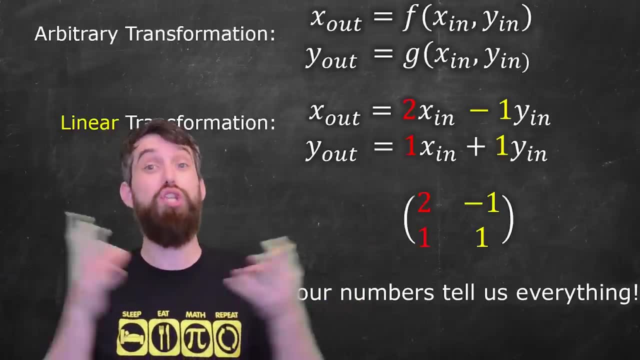 But then the algebraic world has to go to a straight line and the origin to itself. And then the algebraic constraint was that any of the input variables, like the x in, has to appear as only that to the power of 1.. And then what's quite magical is that these two different constraints really seem to be. 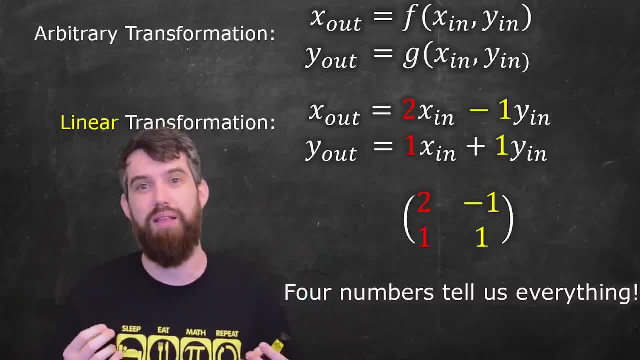 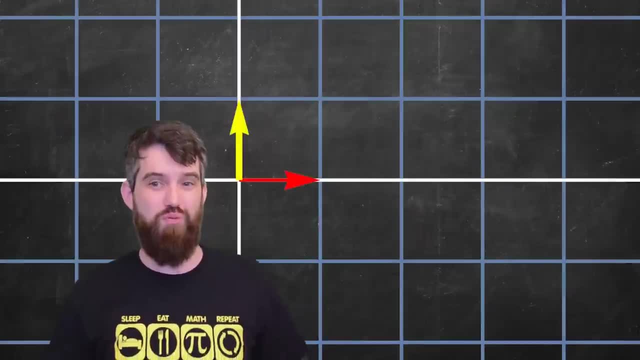 the same thing, That they're two different sides of the same coin. So I want to show you one more interesting way that we can relate something algebraic and something geometric. So remember this particular transformation that we had, This one that we've been looking at and we've seen are two vectors. 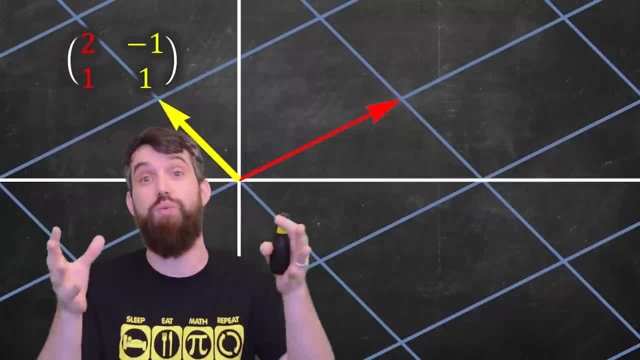 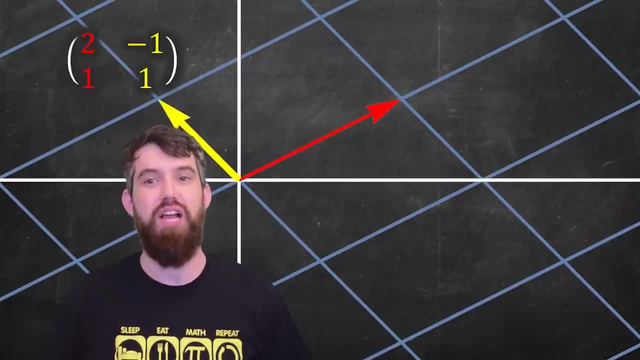 And we saw that that was associated with these four numbers: The 2, 1, minus 1, 1.. Well, what about the transformation that sort of undoes it, This transformation, The one that takes those vectors and puts them back to where they began?